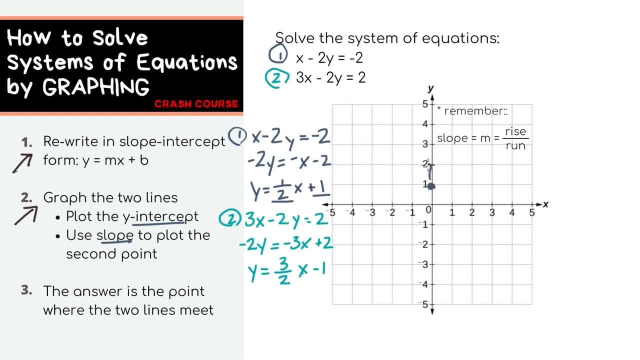 From here, the rise is positive 1,, so let's go up 1, and the run is positive 2,, so let's go to the right by 2.. Now connect the dots to get the full line. We'll do the same to our second equation. 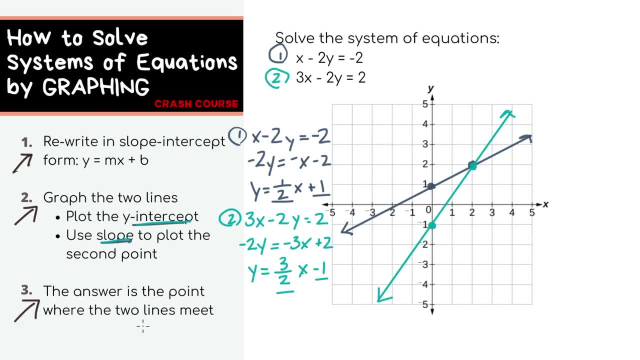 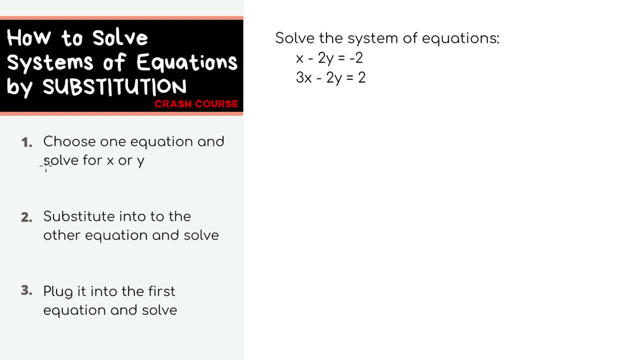 Step number three, you'll notice that our line crosses at the point 2, 2.. So this is actually our answer: x equals 2 and y equals 2.. So let's check out the next step In order to solve systems of equations through substitution. 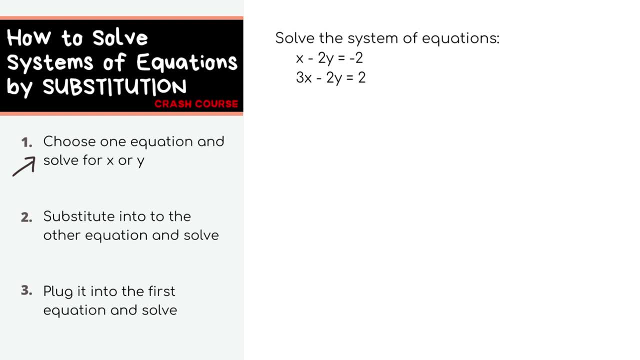 you first need to solve for one of the variables. Obviously, choose the one that's easiest to solve for. I see here that we can easily solve for x in the first equation, because there's no coefficients, no mess. Just add 2y to both sides of the equation and you'll get x equals negative 2 plus 2y. 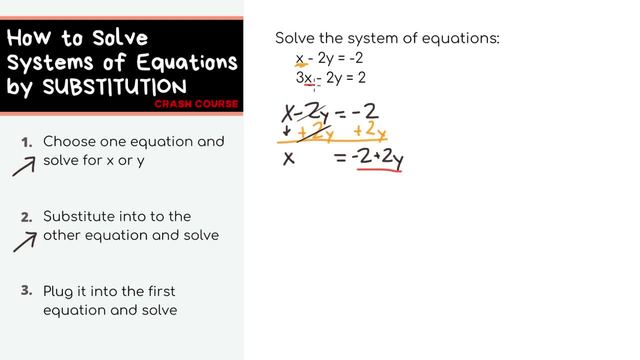 Next step: substitute what you need to solve. you just got into the other equation. you'll end up with this expression: when you substitute for x, Let's distribute, simplify and solve. We'll end up with y equals 2.. Final step: plug what you just got back into the equation from step one. 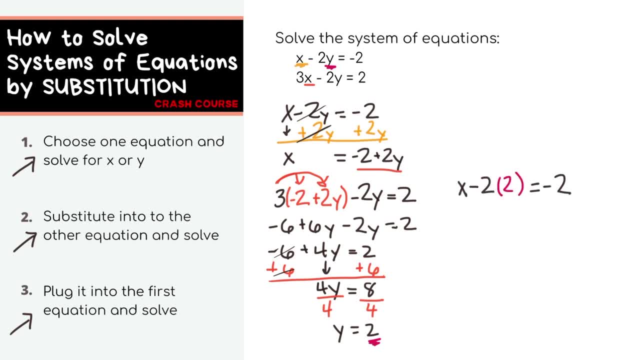 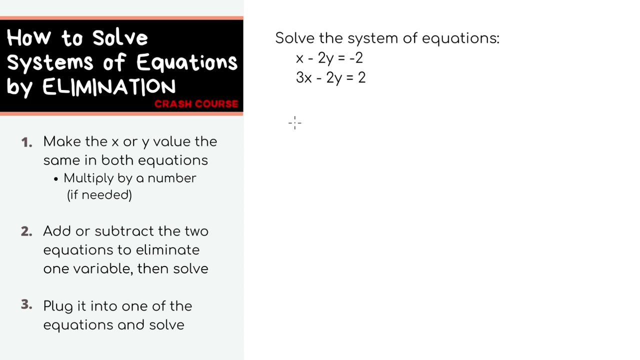 We'll get x equals negative 2 plus 2 times 2 and end up with x equals 2 when we simplify, That's again our final answer: x equals 2 and y equals 2.. Last method: elimination. In order to solve systems of equations through elimination, 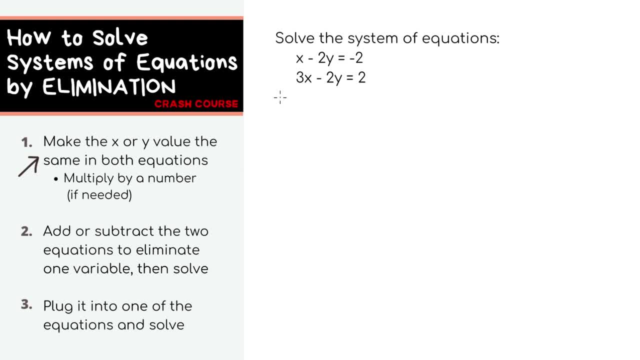 you first look at the two equations and choose either x or y to eliminate. For the variable you choose, you have to make the coefficients of the two equations equal to, or equal to zero, Or the number in front of the variable, the same in both equations. 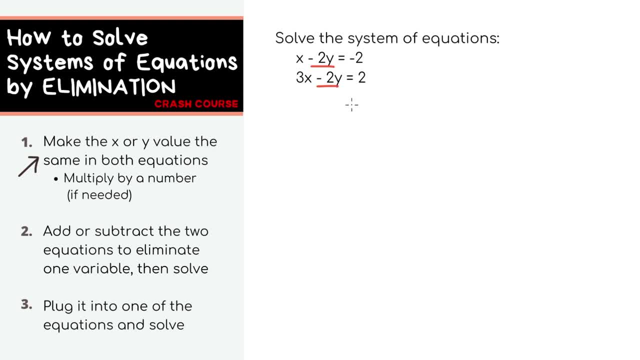 Here we got lucky and both equations already have negative 2y, so I'm going to choose y. For some reason, if we chose x to eliminate, we have to multiply both sides of the first equation by 3, so that both equations have 3x. 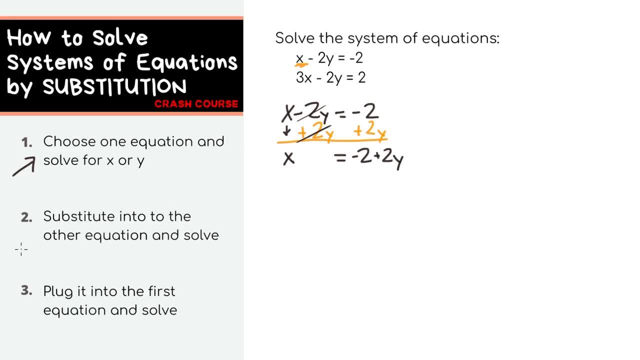 no mess. Just add 2y to both sides of the equation and you'll get x equals. and you'll get x equals 2y plus 2y- what you just got into the other equation. you'll end up with this expression when you substitute for x. Let's distribute, simplify and solve. 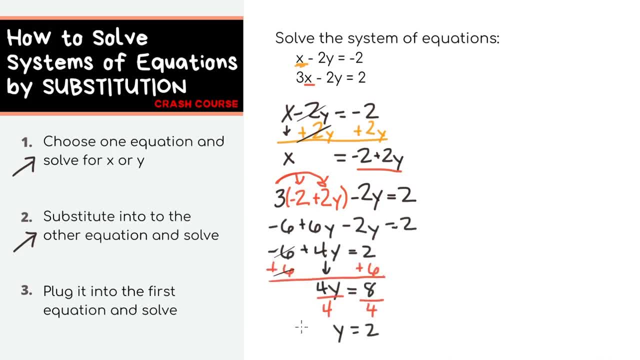 We'll end up with y equals 2.. Final step: plug what you just got back into the equation from step 1.. We'll get x equals negative 2 plus 2 times 2 and end up with x equals 2 when we simplify. That's again our final answer: x equals 2 and y equals 2.. 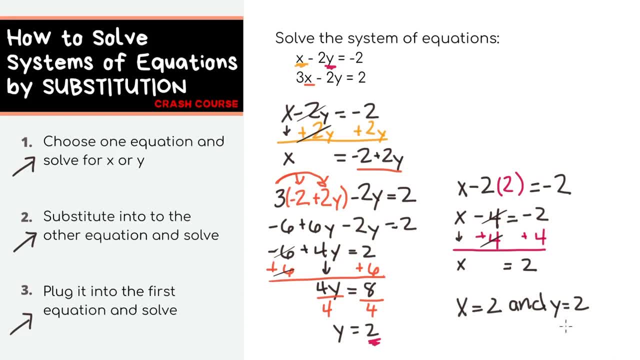 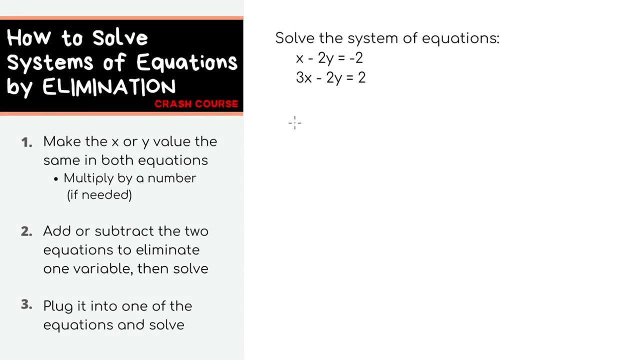 Last method: elimination. In order to solve systems of equations through elimination, you first look at the two equations and choose either x or y to eliminate. For the variable x equals 2, when we simplify, that's again our final answer: x equals 2 and y equals 2.. 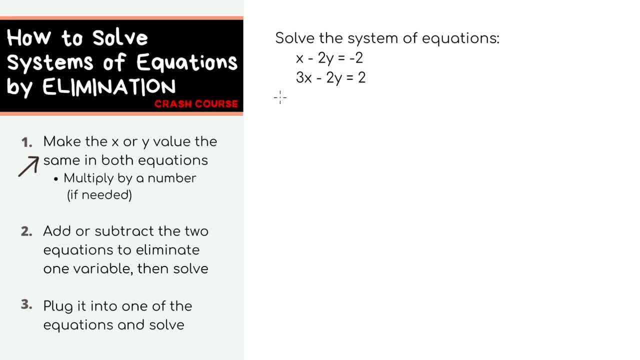 you choose, you have to make the coefficients, or the number in front of the variable, the same in both equations. Here we got lucky and both equations already have negative 2y, so I'm going to choose y. For some reason, if we chose x to eliminate, we have to multiply both sides of the. 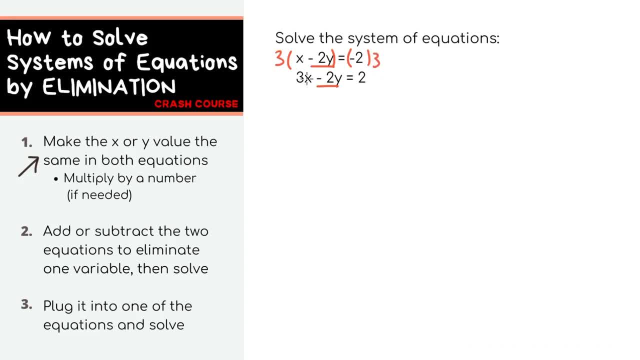 first equation by 3, so that both equations have 3x Next up. since both equations have negative 2y, we should subtract the two equations to eliminate the y variable. x minus 3x is negative, 2x negative 2y minus negative 2y equals 0, which is exactly what we wanted to do. We've eliminated 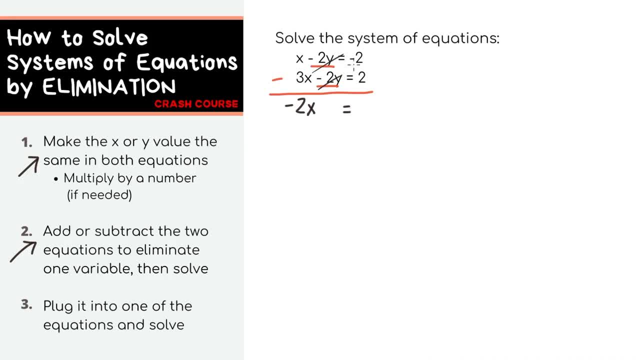 the y variable and negative 2 minus 2 equals negative 4. Dividing both sides by negative 2, we'll get x equals 2.. Last step: plug in x equals 2 into one of the equations, It doesn't really matter which one. 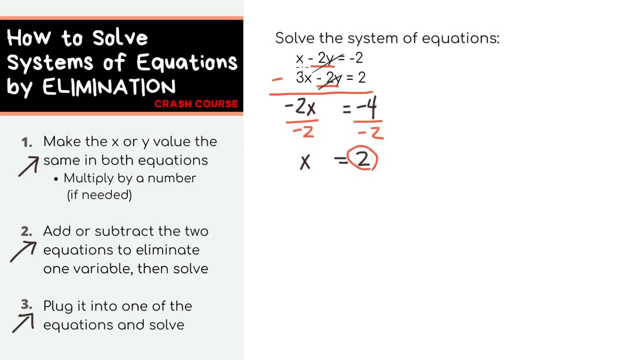 just choose the one that's easiest. I'll do the first equation: Simplifying. you'll get y equals 2.. So again, that's our answer: x equals 2 and y equals 2.. Thanks for watching this crash course on solving systems of equations.